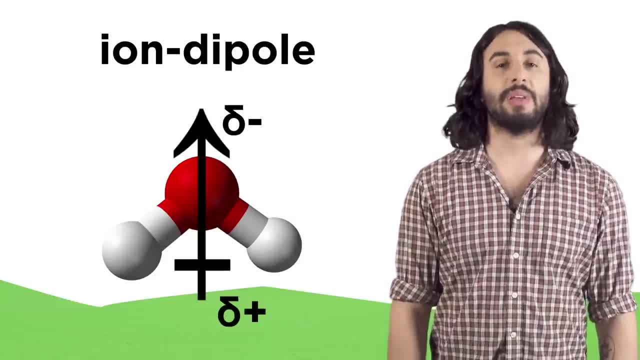 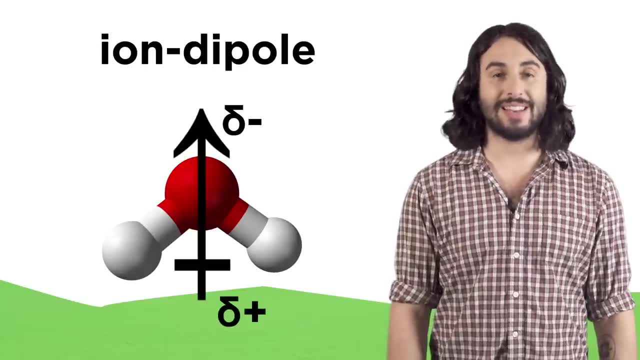 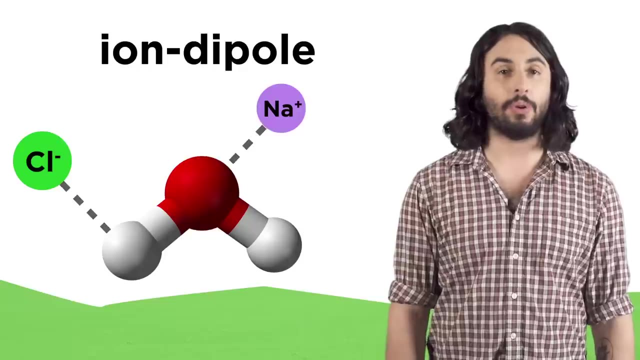 dipoles can make electrostatic interactions because the partially negative side is attracted to positive charges and the partially positive side is attracted to negative charges. so when sodium chloride dissolves in water, the sodium ions make ion-dipole interactions with the negative side of water's dipole. 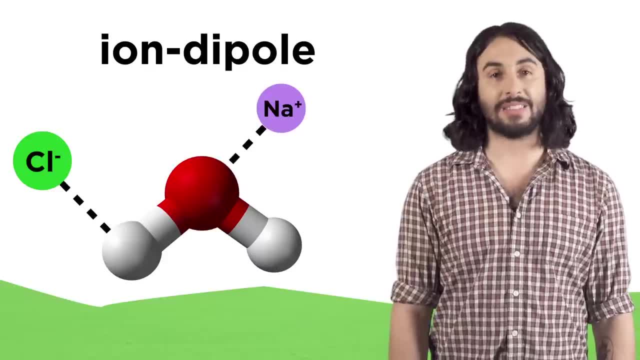 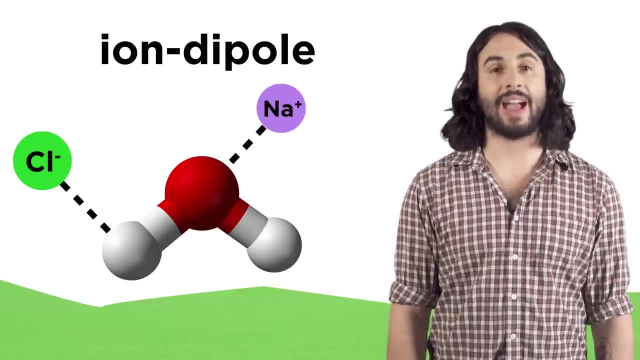 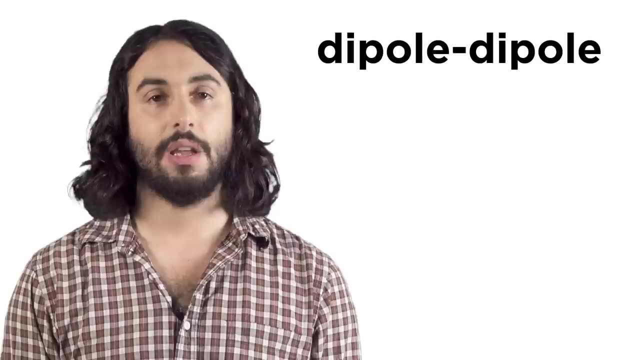 and the chloride ions make ion-dipole interactions with the positive side of water's dipole. each ion can make several of these interactions, which store a lot of energy, which is why sodium chloride will dissociate in water in the first place. next we have dipole-dipole interactions. 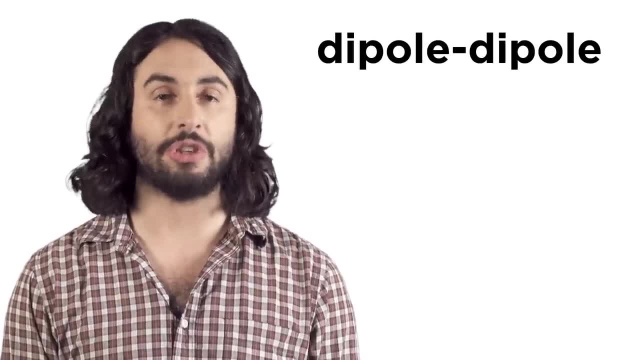 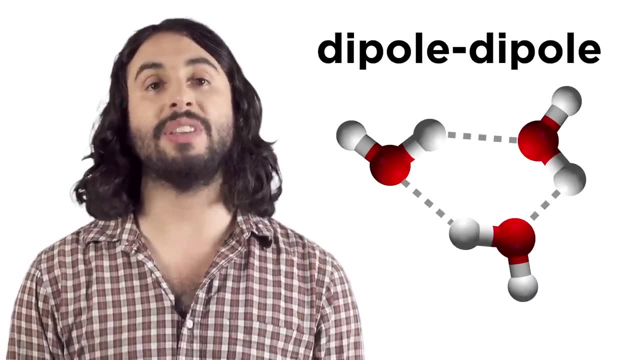 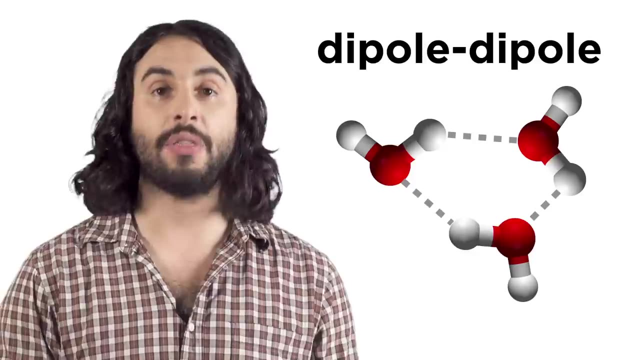 as you can guess, this is when dipoles interact with each other, as with pure water, when, in liquid form, water molecules will move in such a way so as to always be making electrostatic interactions between the negative end of one dipole and the positive end of another dipole. 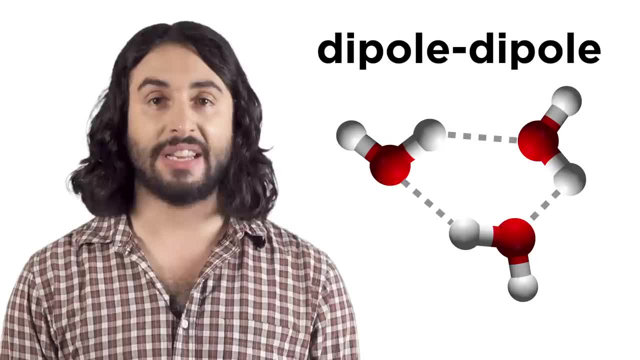 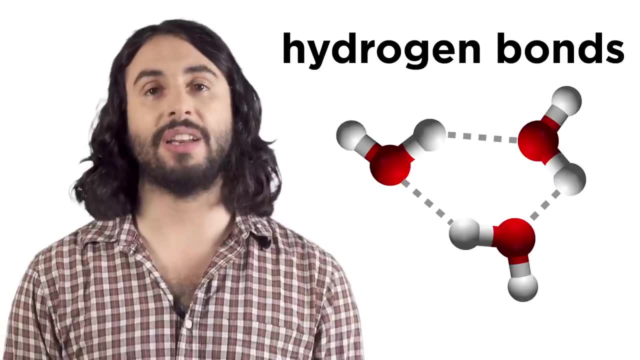 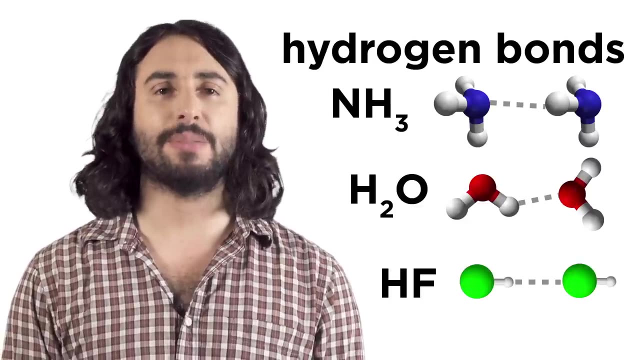 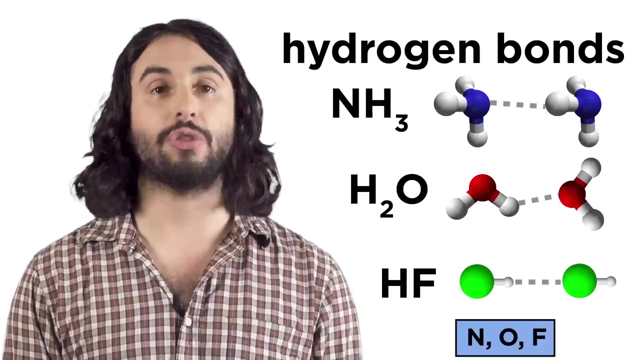 in this case, these dipole-dipole interactions qualify for a special title: hydrogen bonds. this is when dipoles generated by NH, OH or FH bonds interact with each other. these are just especially strong dipole-dipole interactions. they are especially strong because these are the most electronegative elements. 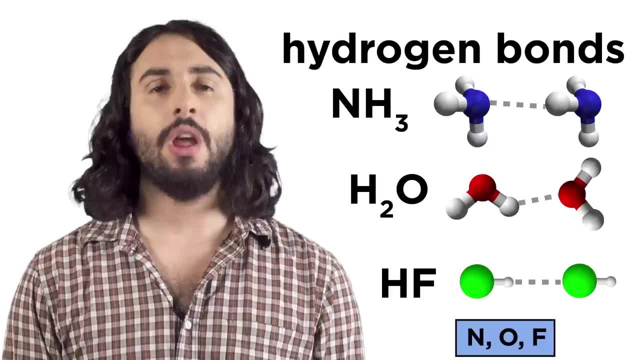 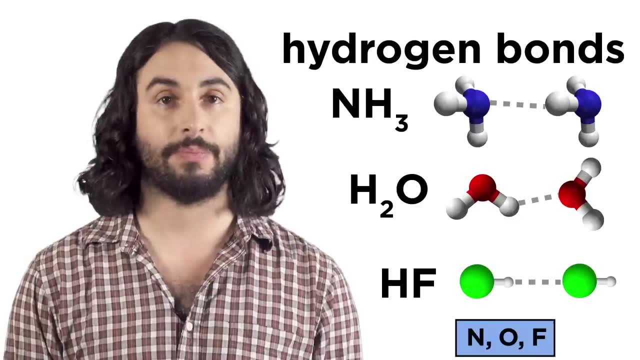 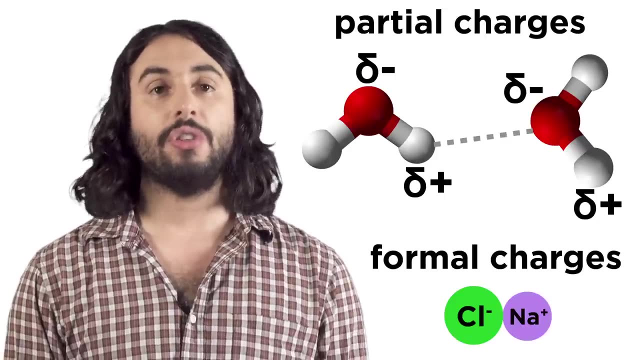 so they will create the most strongly polarized bonds, resulting in a very strong dipole and therefore very strong dipole-dipole interactions. we can almost think of partial charges as some fraction of a formal charge. so the greater the partial charge, the stronger the interaction. 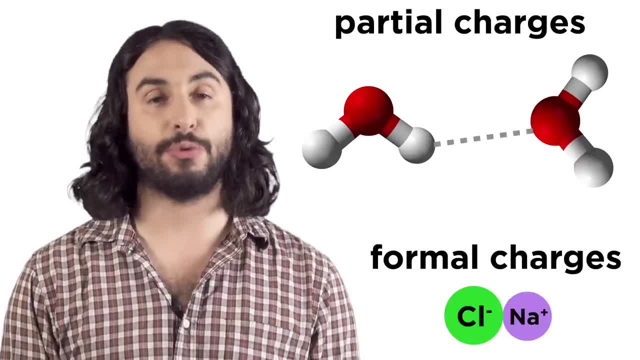 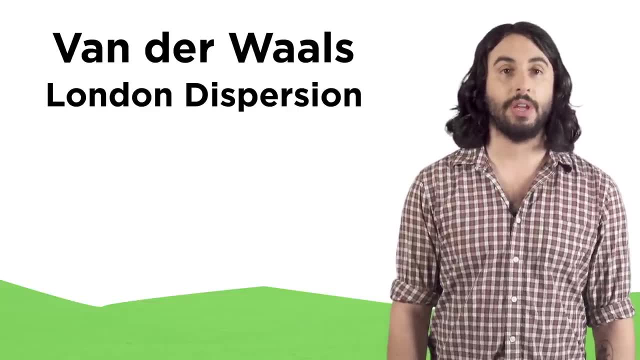 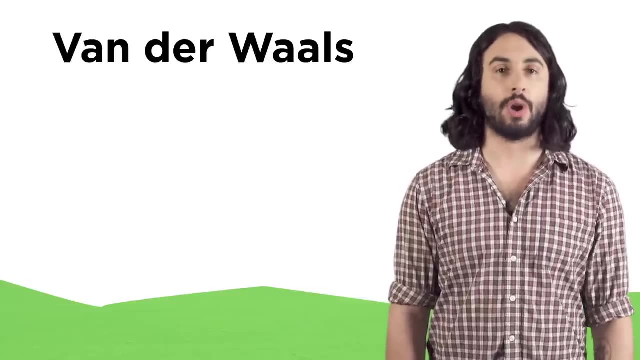 though never quite as strong as interactions between formally charged particles. lastly, we have the van der Waals or the London dispersion force. these names refer to the same force and are completely interchangeable, so I will arbitrarily refer to them as van der Waals forces. this is the consolation prize of the intermolecular forces. because any substance can do it. only ions make ion-ion interactions and only covalent molecules with a dipole can make dipole-dipole interactions. but absolutely anything can do, van der Waals, for example. take a look at helium. helium is a noble gas and due to a full valence shell, it does not make bonds with other atoms. 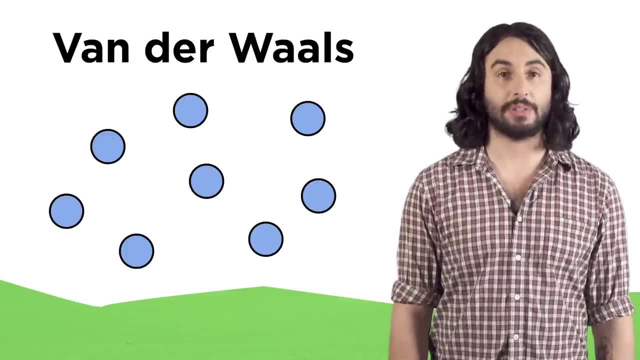 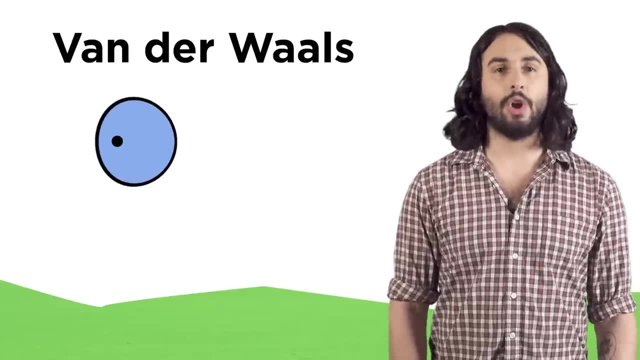 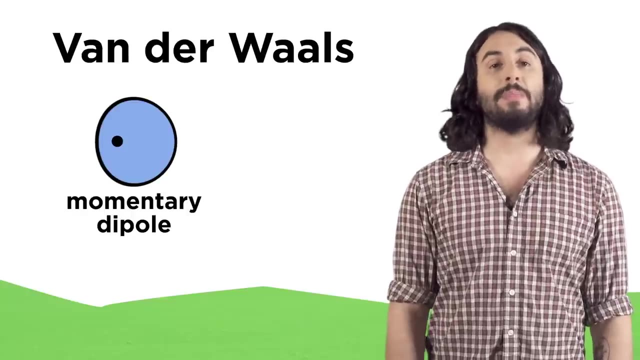 so a sample of helium is just a bunch of helium atoms. well, the electron cloud around a helium atom will at any time be slightly lopsided or skewed towards one direction. this will result in something called a momentary dipole. this means one side of the atom is ever so slightly partially negative. 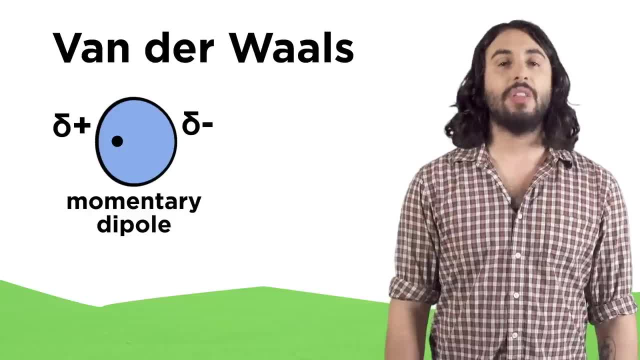 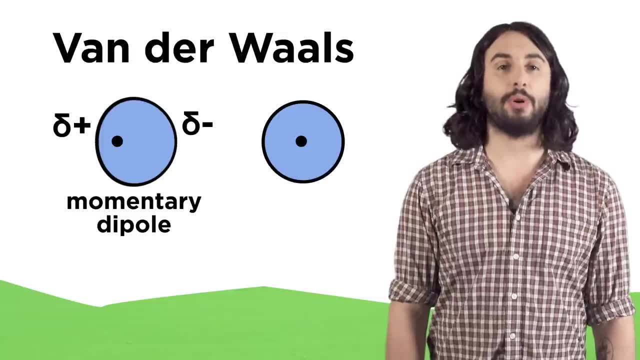 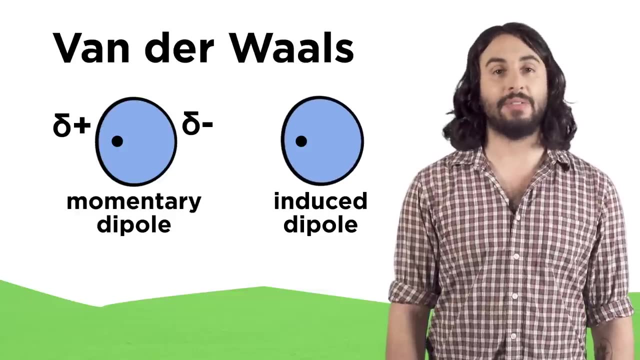 and the other side is slightly partially positive. this is much weaker than a formal dipole, but it still exists and can be measured. if a momentary dipole approaches another atom, it can generate an induced dipole, meaning the slight partial negativity repels this electron density over to the other side of the atom. 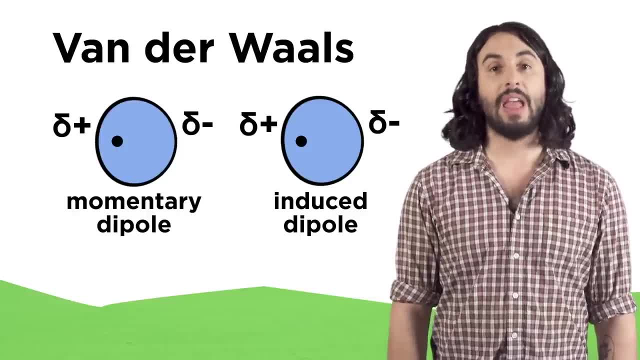 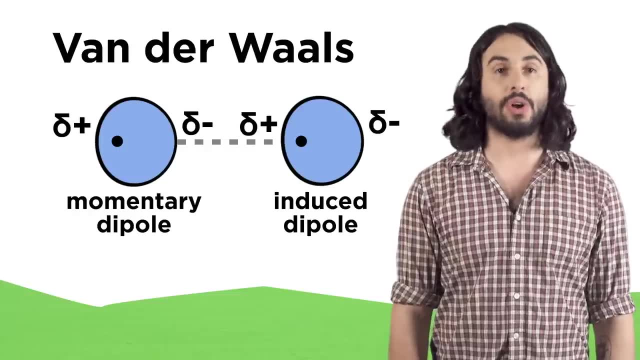 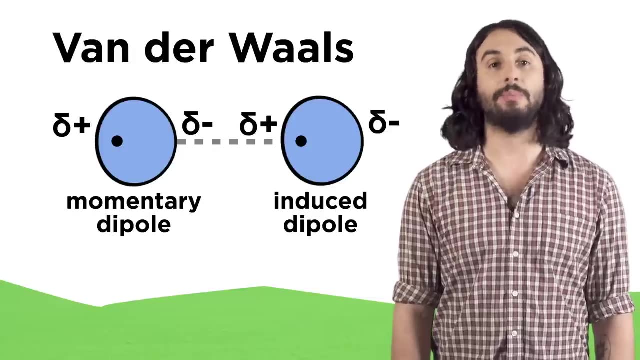 so it will also have a slight dipole and then there can be a momentary dipole-induced dipole interaction. that is the van der Waals force. this is a weak and fleeting attraction, but this is all that monoatomic species and nonpolar covalent compounds can do. 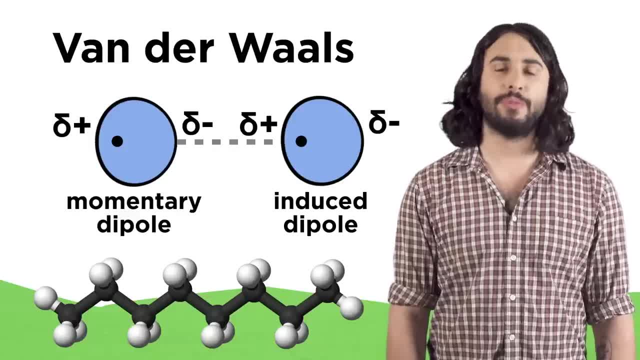 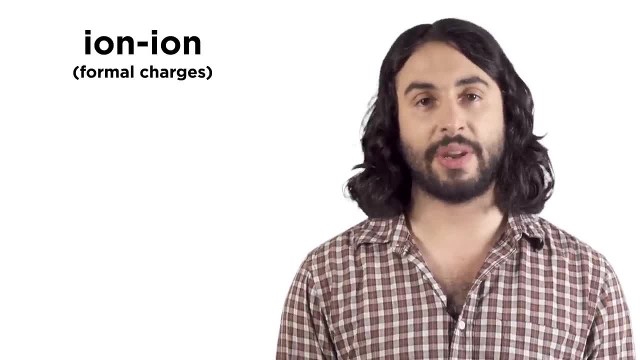 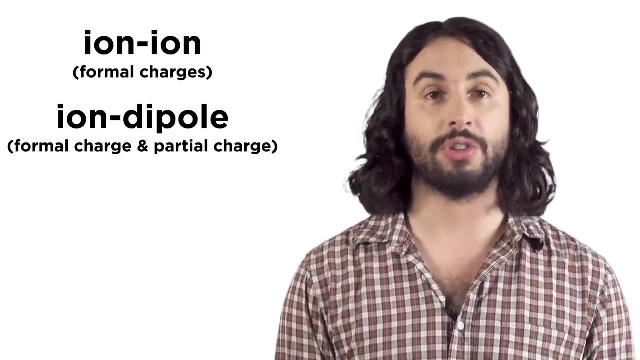 and for very large molecules, like some hydrocarbons, the force can become significant. so the ion-ion force is strongest because it involves interactions between formally charged particles. ion-dipole is next because it involves a formal charge and a partial charge, then dipole-dipole, which is between partial charges. 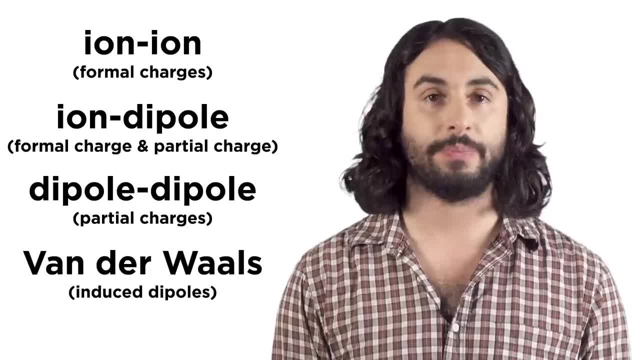 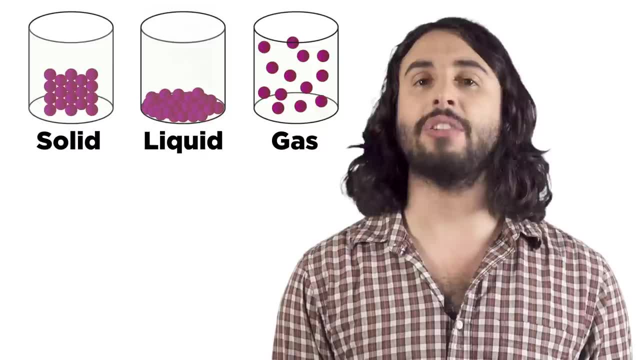 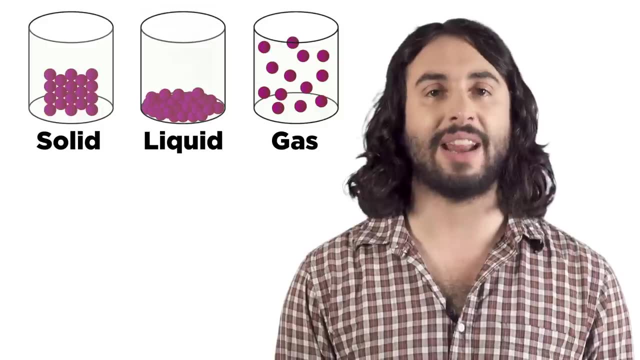 and van der Waals, which is between tiny induced dipoles, to see how intermolecular forces dictate phase change. let's do a thought experiment first. recall that a solid's particles are rigidly packed and not moving. a liquid's particles are moving, but they are still close together and interacting. 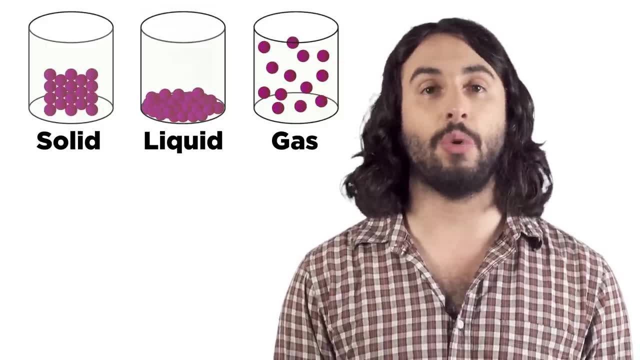 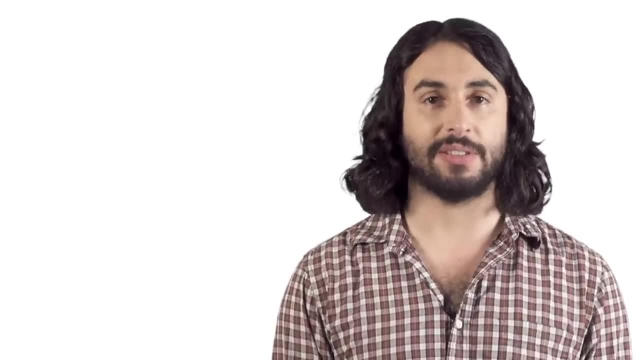 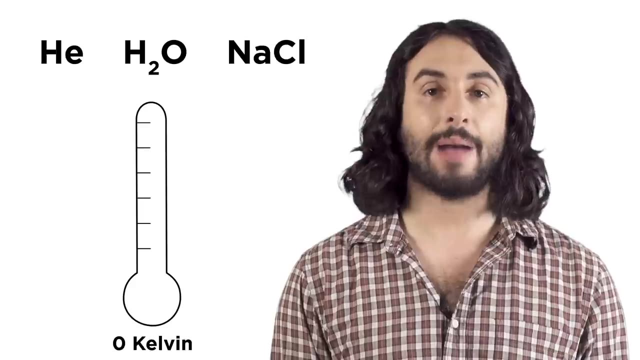 gaseous particles are moving and they are far away from each other, so compared to liquids, they basically don't interact. so let's pretend we have three substances: helium, water and sodium chloride. we will place them at zero kelvin, or absolute zero, which is the lowest temperature possible. 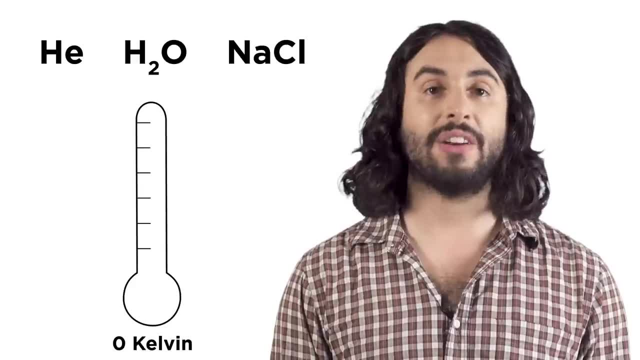 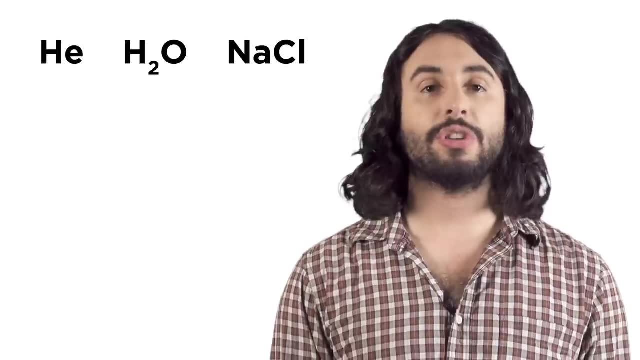 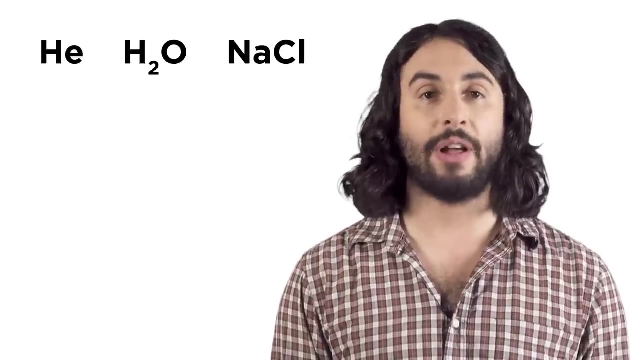 a complete absence of heat energy, where there is no energy available for motion. here everything, even helium, is a solid. in order to go from the solid to the liquid, to the gas phase, heat energy has to go into the sample and overwhelm the intermolecular forces that are occurring. 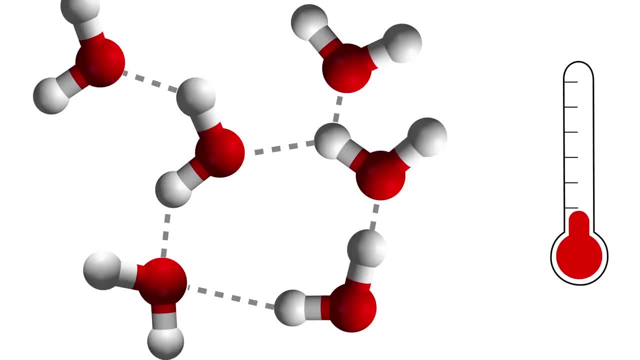 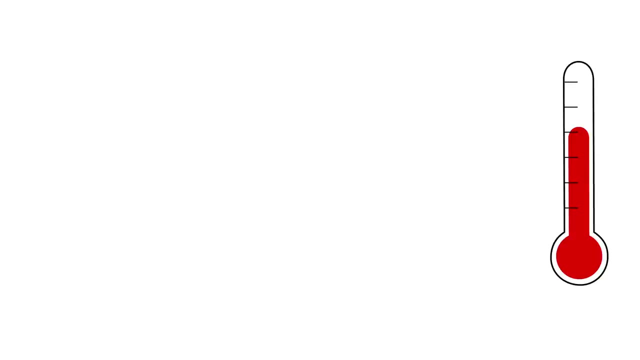 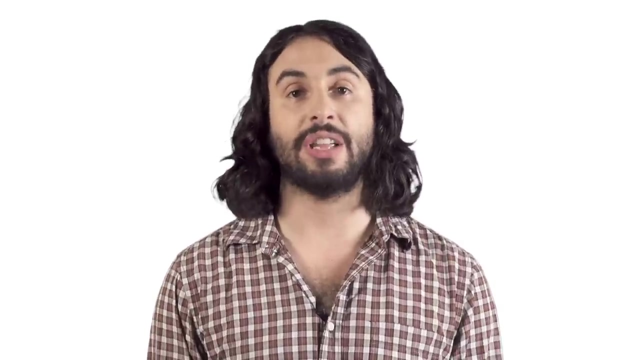 in a liquid there is some energy stored in electrostatic interactions, and whatever amount that is, that is precisely the amount of heat energy that has to be provided to liberate the molecules into the gas phase, where they are not interacting and not storing energy, because nature will not tend to go to a higher energy spontaneously. 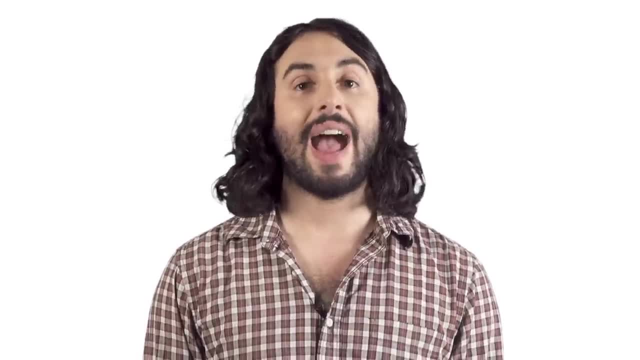 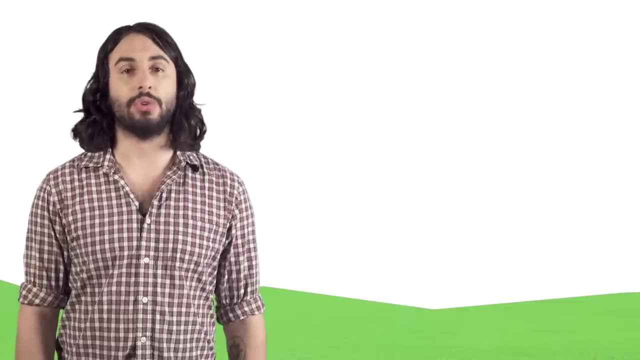 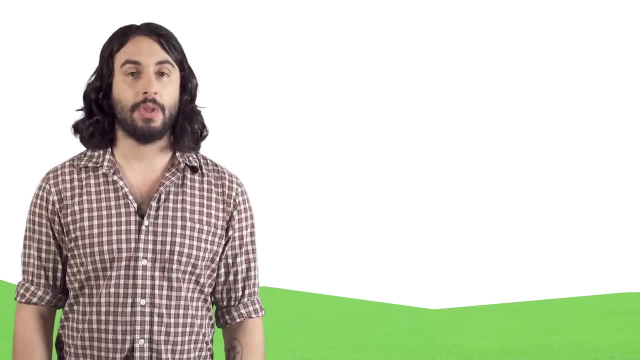 so the energy stored in these interactions has to be provided in some other way. this means that the stronger the forces between the molecules are, the more heat energy we will have to provide to melt and boil the sample. so let's take our three substances slowly, raise the temperature. 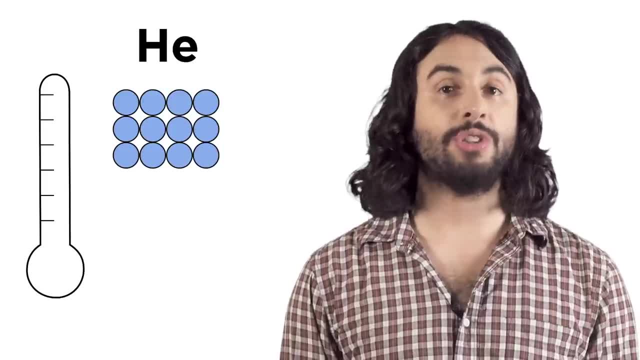 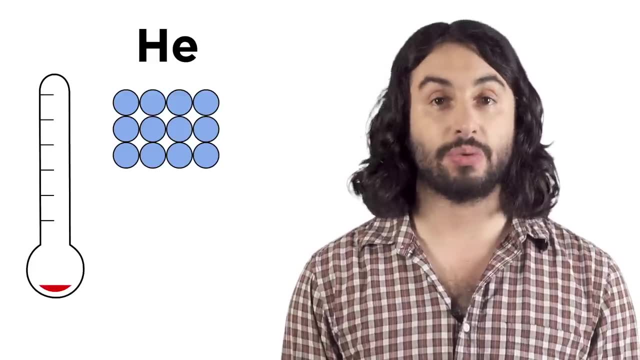 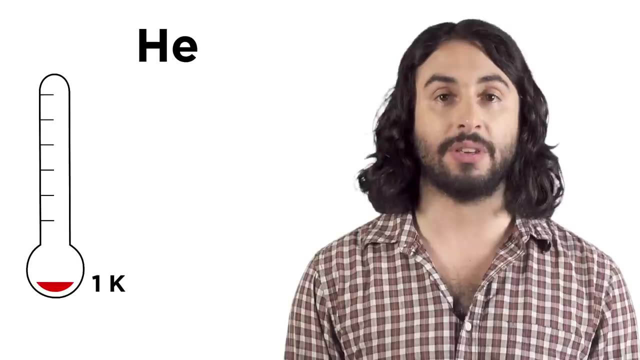 and see what happens. helium, as it is only participating in incredibly weak van der Waals forces, needs only a miniscule amount of heat energy to disrupt these weak interactions. that's why helium will melt and boil at barely one degree above absolute zero. water, on the other hand, is participating in strong dipole-dipole interactions. 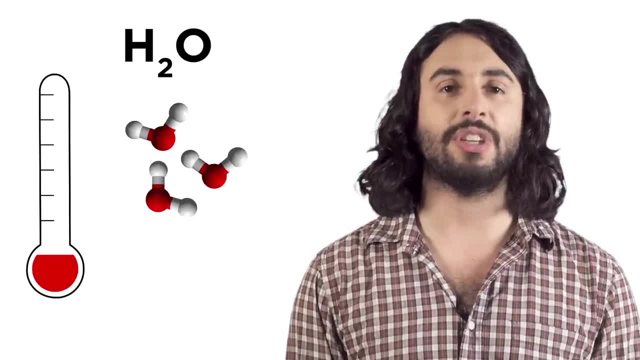 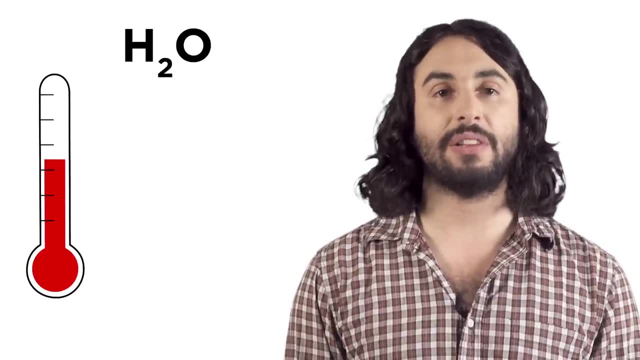 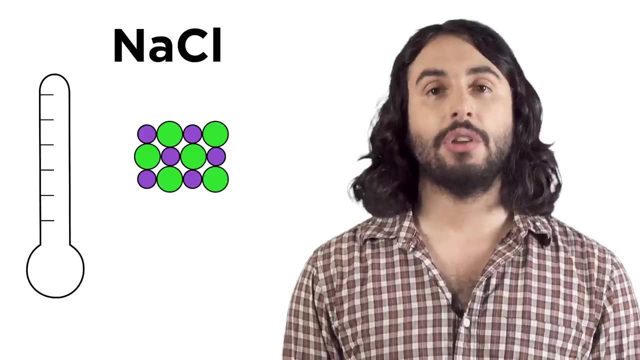 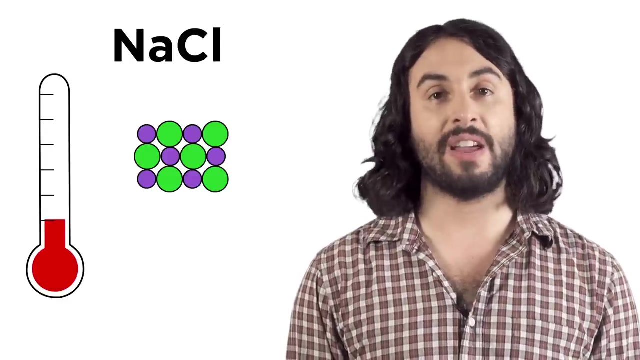 called hydrogen bonds. there is a significant amount of energy stored in these interactions, so we will need considerable heat energy to overcome them. water melts and boils at 273 and 373 kelvin respectively. lastly, sodium chloride is making extremely strong ion-ion interactions, so it will take a huge amount of energy to melt and boil this solid. 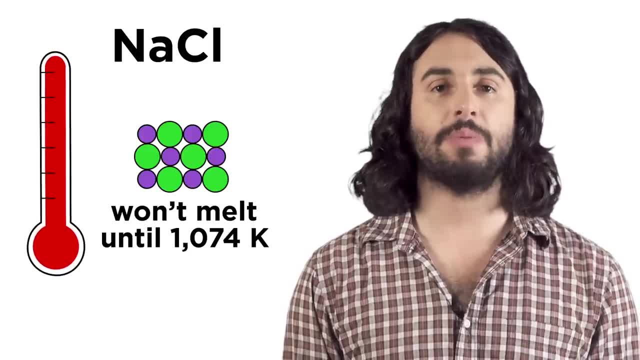 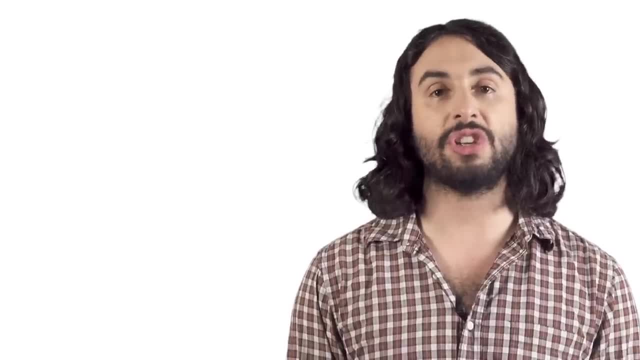 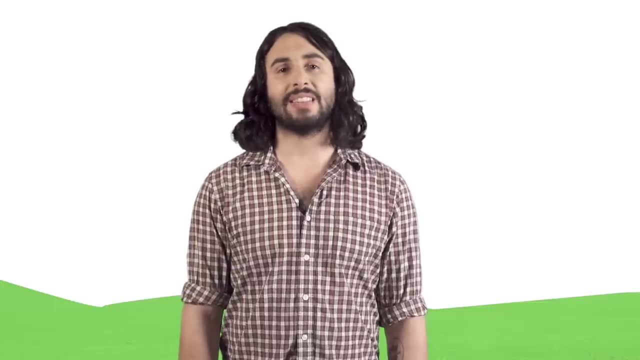 it melts at 1074 kelvin, which means there's a lot of energy stored in the ion-ion forces. we can use this information to decide which of a given set of compounds might have the highest boiling point. when we ask this question, we are really asking. 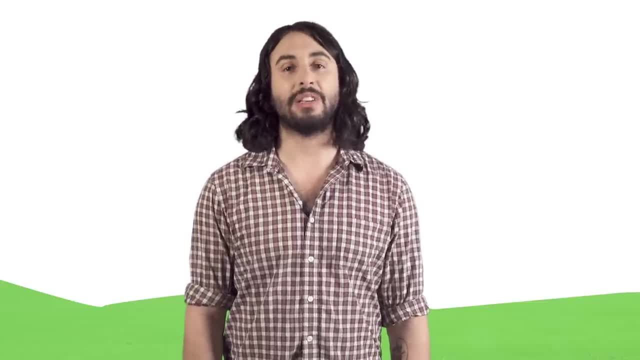 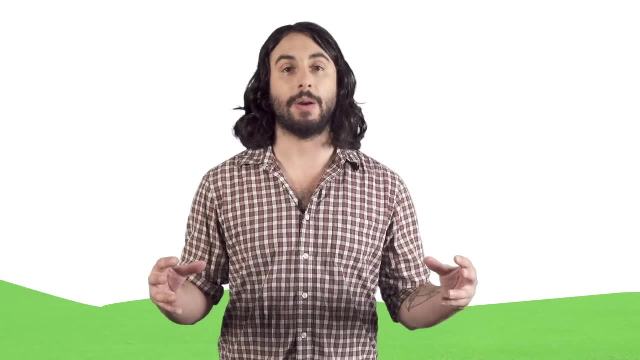 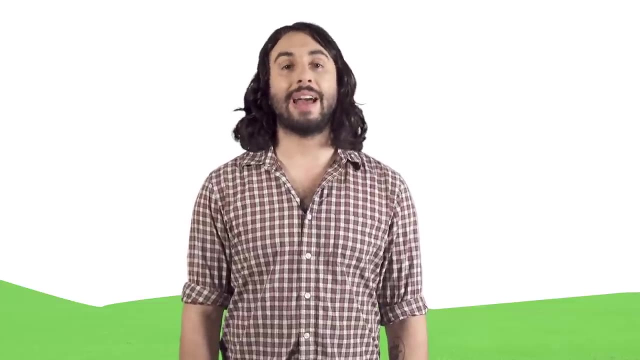 which compound is generating the strongest intermolecular forces. the stronger they are, the more heat energy. we will need to pull the molecules apart and put them in the gas phase so they will boil at higher temperatures. we need to be able to look at a molecule and decide what kind of interactions it will make.